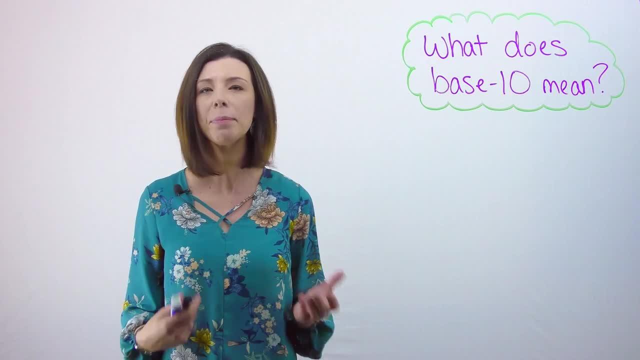 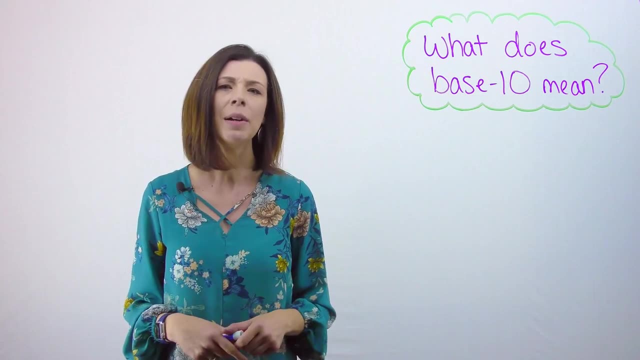 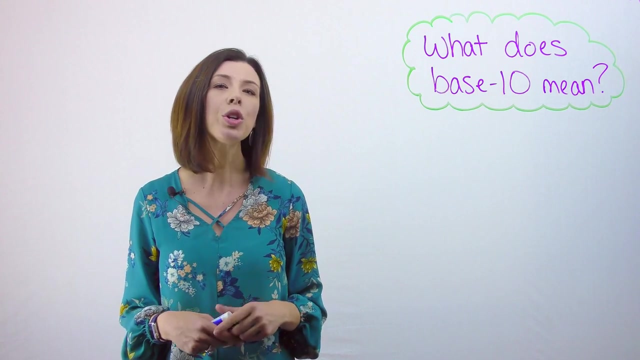 Part of understanding place value is understanding our base 10 system. So that leads me to think: what is base 10?? What does that even mean? When I ask you what base a number is in, what am I referring to? This video is going to give you an introduction to what I mean by that. 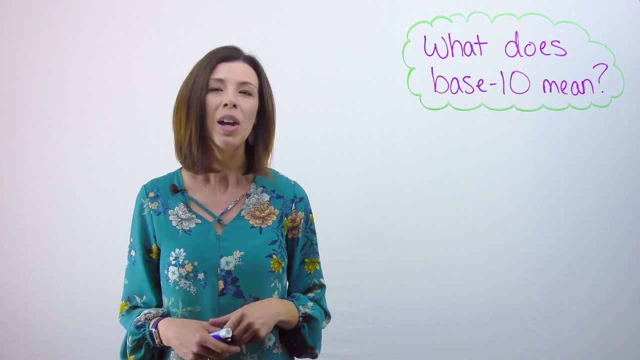 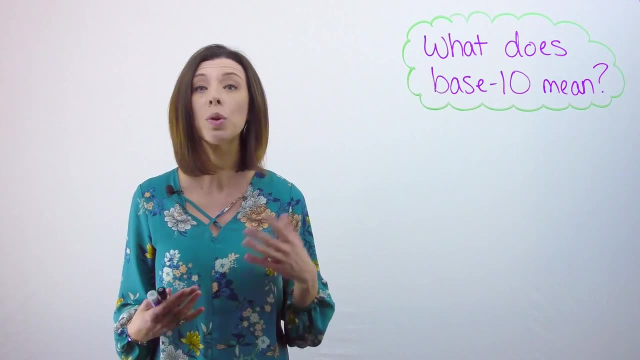 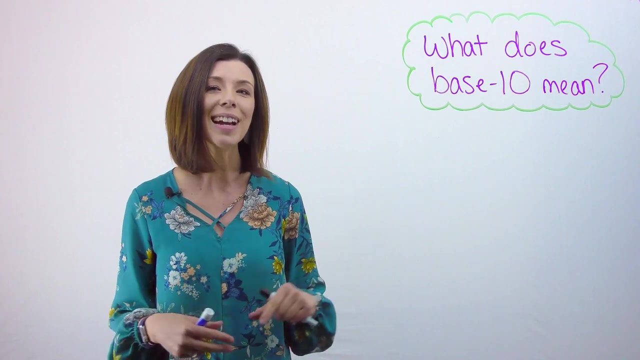 and help you to better understand our base 10 system. So you might remember that in maybe kindergarten first grade, you remember hearing that every number was broken down into ones tens, one hundreds. This is coming from base 10.. So our base system In our society. 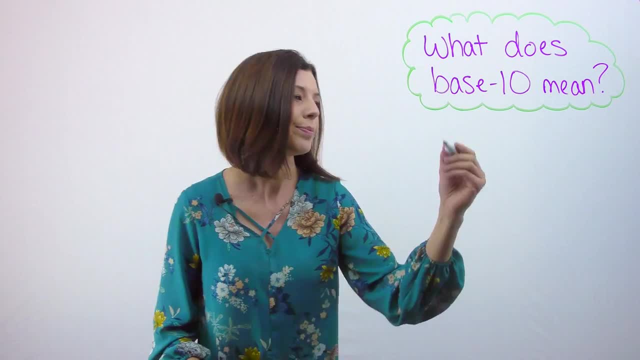 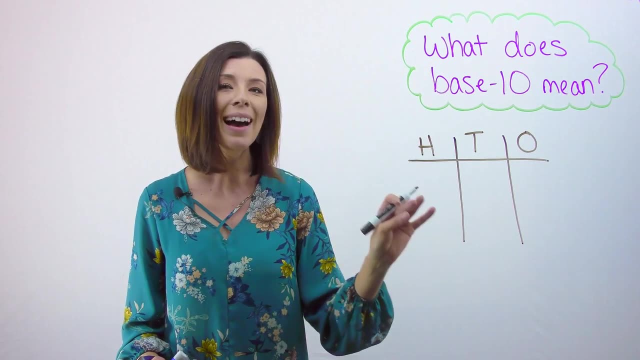 we use a base 10 system. Here's exactly what that means. Maybe you've seen a ones, tens and hundreds place value chart before. The math behind this, though, is where we look at our bases, So when I think about the ones place really 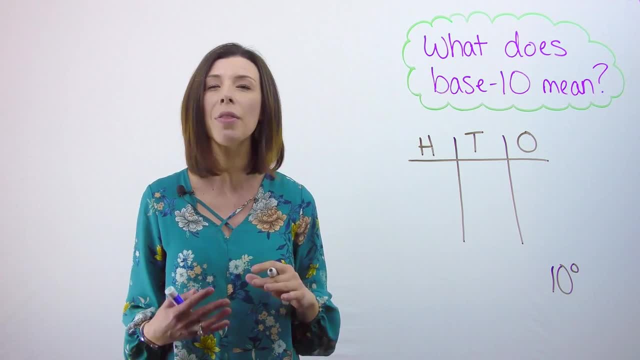 I'm thinking about the ones place. So when I think about the ones place, I'm thinking about the ones place. So when I think about the ones place, I'm thinking about the ones place. So when I'm thinking about the ones place, I'm thinking about ten to the power of zero, because we know. 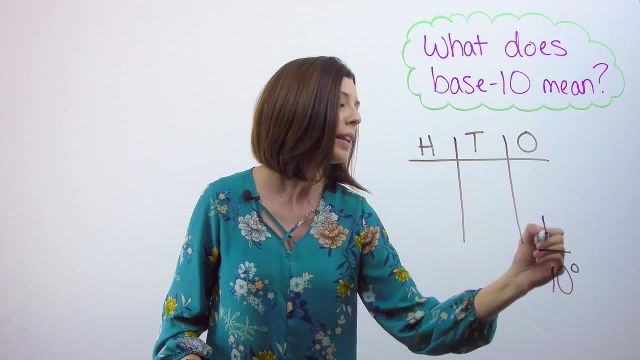 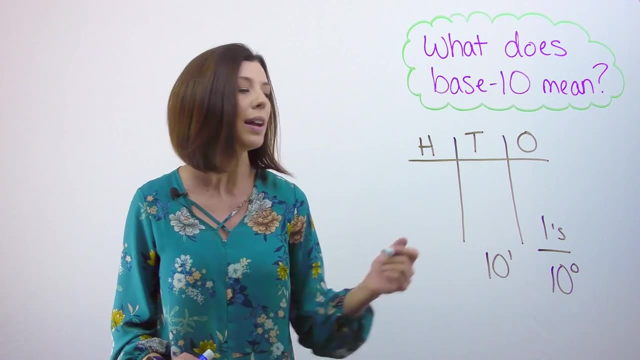 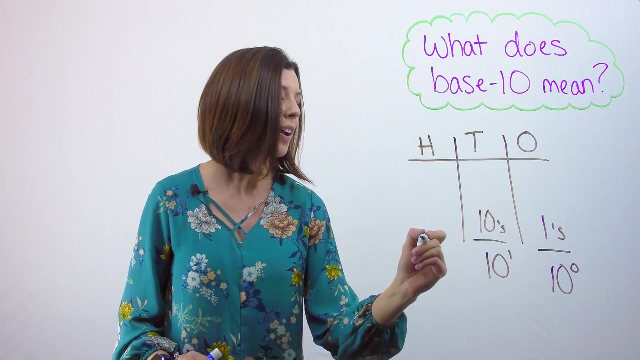 that anything to the power of zero is one. This is where I get my ones place, Likewise my tens place. I know that I get that from ten to the power of one. Ten to the power of one is ten. Hence we call it the tens place. If I keep going, I get to the hundreds, and I know that I get ten squared. 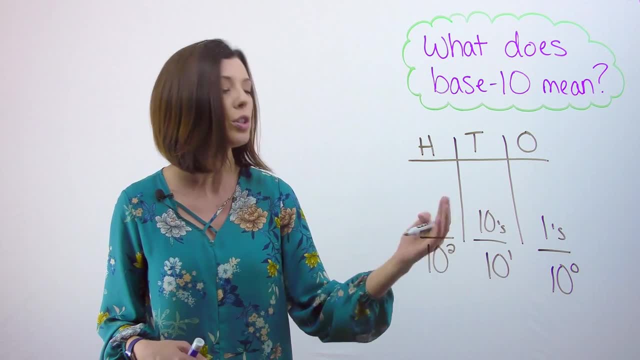 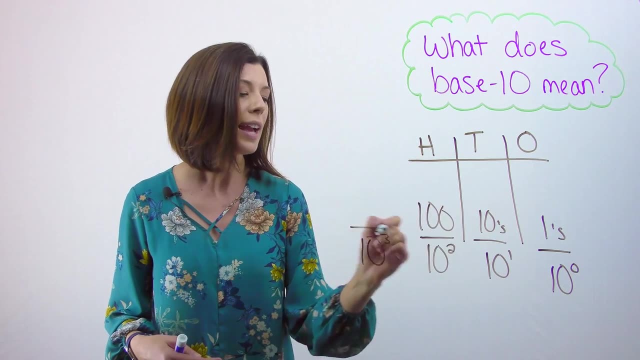 Are you seeing a pattern? I have to the power of zero, one, two. I can keep going. For the thousands place, I've got ten cubed. So ten squared is one hundred, Ten cubed is one thousand, If you think. 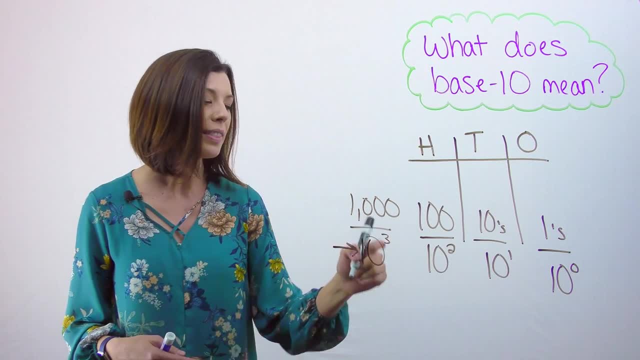 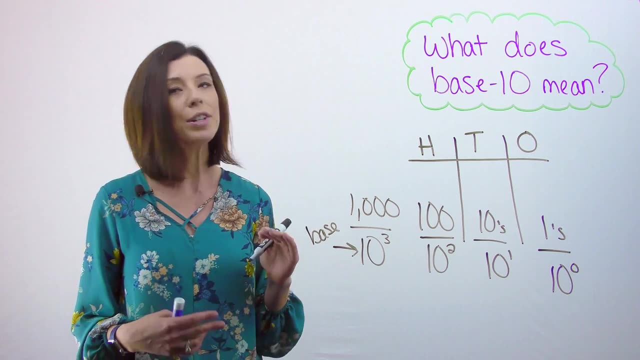 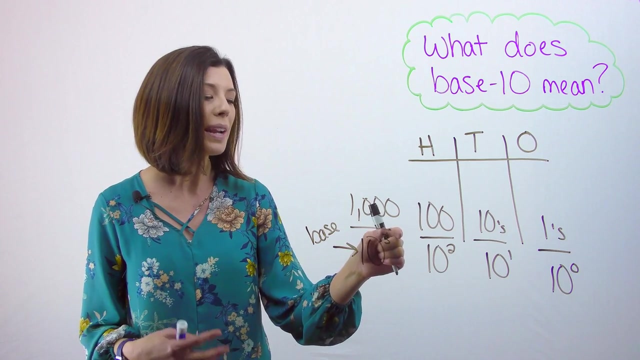 back to exponents. you know that that term right there, this ten piece that's called the base, right We have a base and we have an exponent. So when we talk about base ten, I'm literally talking about what's the base number that we are using to raise to this exponential power. 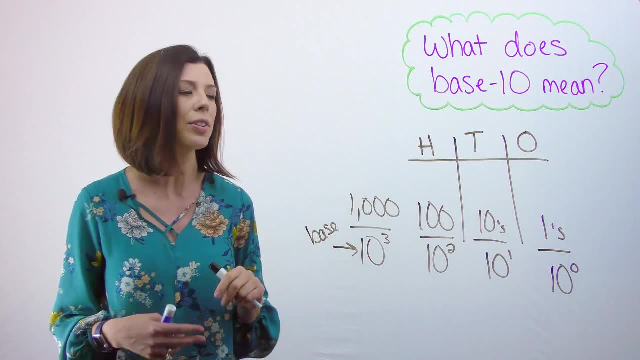 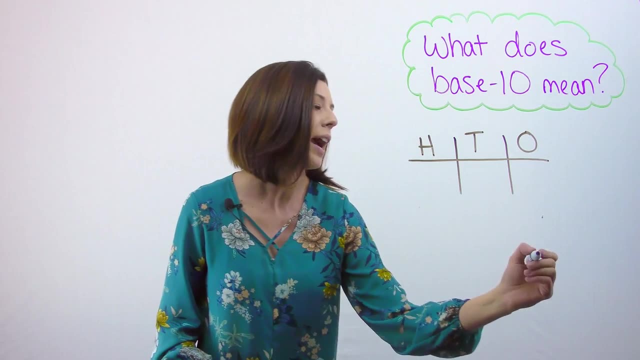 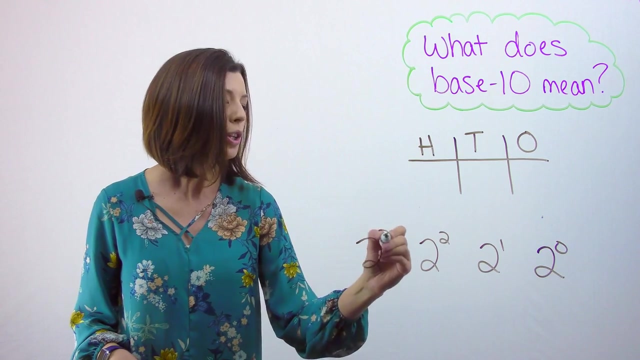 that gives me this number. okay, So let me give you an example. Let's say we were operating in base two. We could write a very similar example. Now, again, you'll notice I have two to the power of zero, two to the power of one, two squared, two cubed. 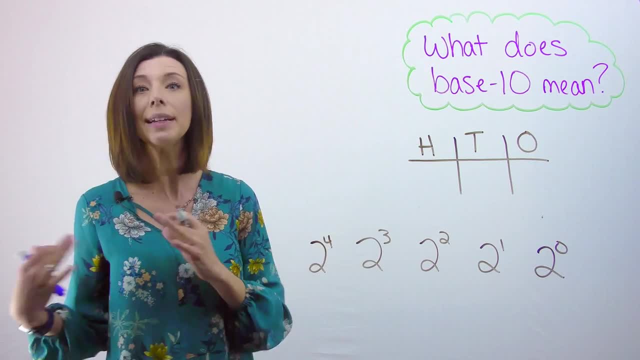 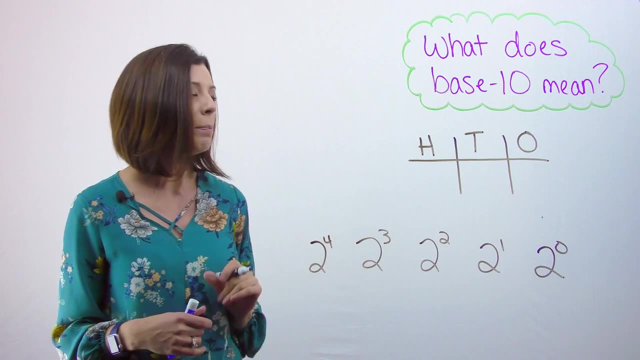 and I could keep going right, Two to the fourth. I don't need to stop. I could keep going forever, But here's where it gets tricky. Now let's go back to our ones tens and hundreds chart. If I'm in base two- and again I know this because there's my base- If I'm in base two, 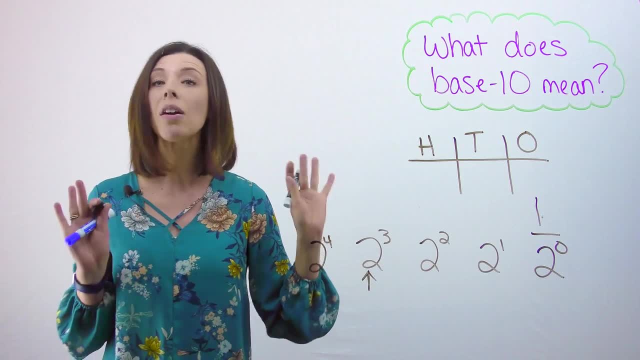 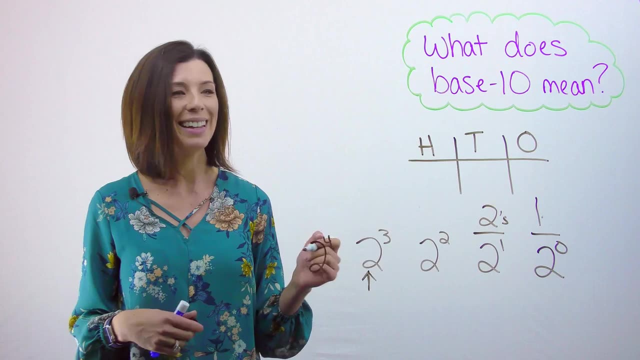 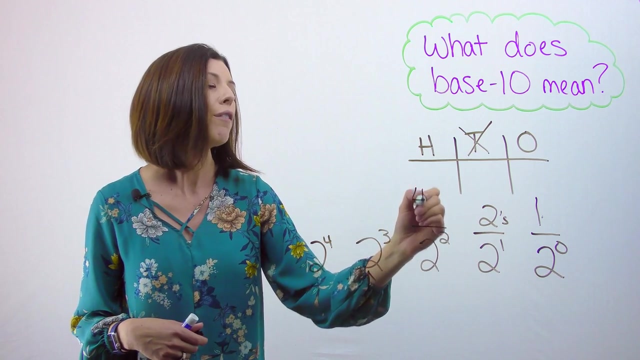 two to the power of zero is still one. I'm still okay calling it ones. However, two to the power of one is two. That's the twos place, not the tens place, although I still have a T there. but you get my point. Two squared is now the fours place, not the hundredths place. 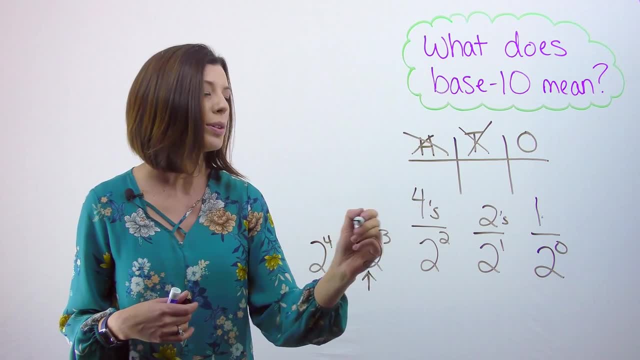 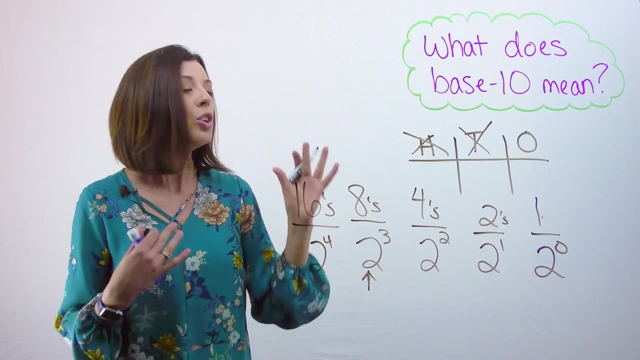 et cetera. okay, So I've got ones: twos, fours, This would be eights, This would be sixteens, I could keep on going right. Notice that I no longer have a tens place, a hundreds place. 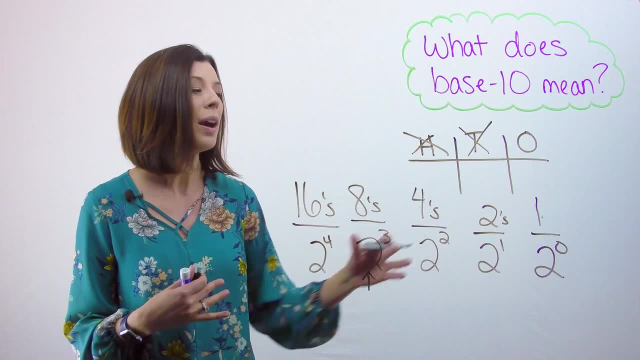 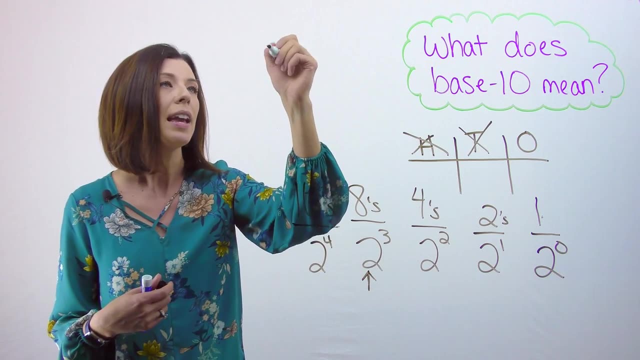 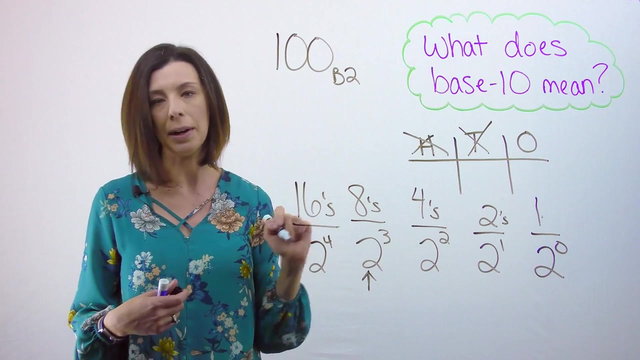 a thousands place. I don't have that anymore. Now in base two I have different named places. Likewise, when I read numbers in other bases, for instance, if I have this number, and when I write numbers in other bases, I write this little like B2 down here: okay, This tells me that I have. 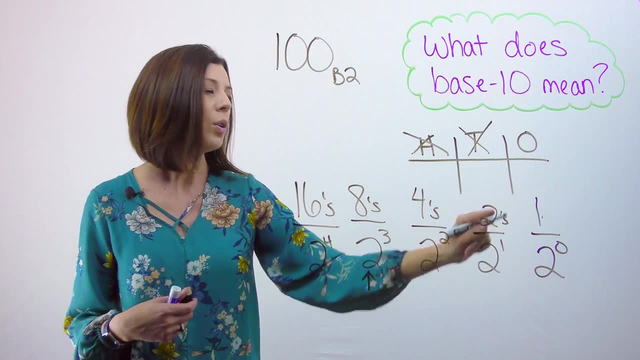 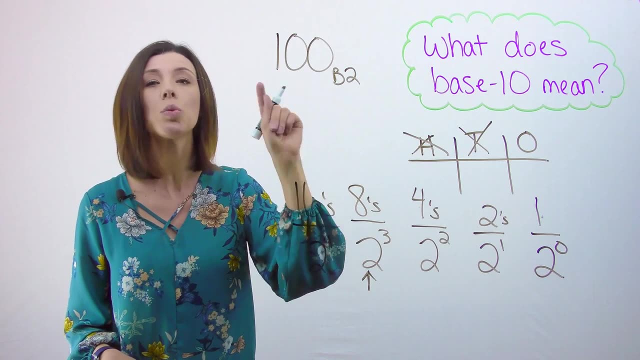 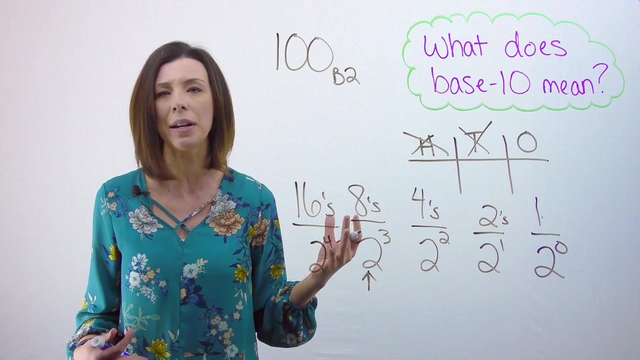 zero ones. I have zero Twos, but I have one four, okay, So I don't read this as 100 base two, I read it as 100 base two. Again, remember, we don't have hundreds anymore in base two, okay, So it wouldn't make sense. for. 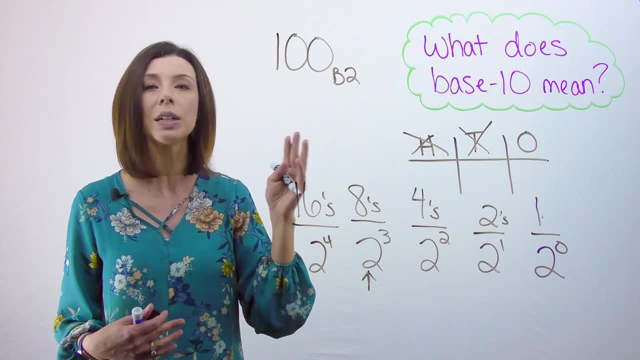 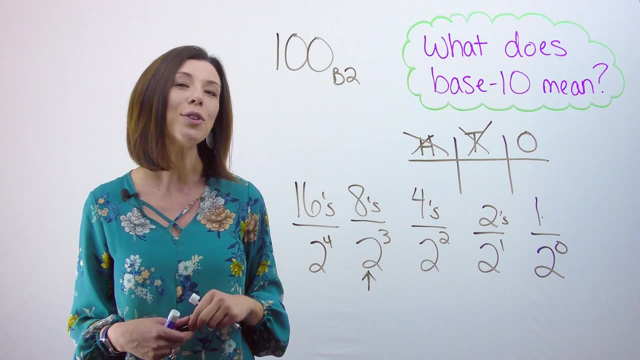 me to call this a 100, though. So what we do is we just say 100, base two: In the next video we're going to look at Egyptians and what system they used, and we're going to see if you can figure out what base they're operating in. So let's get started. 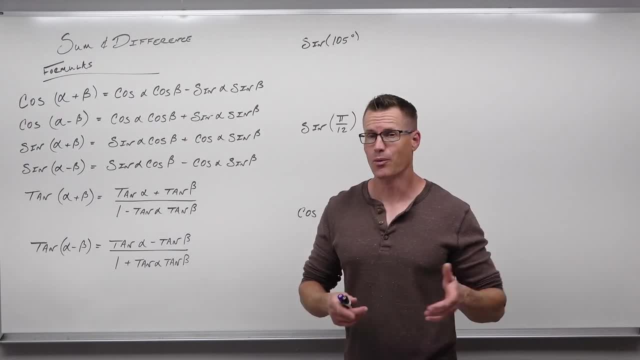 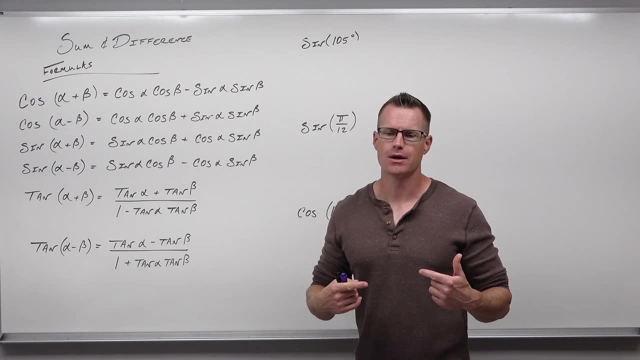 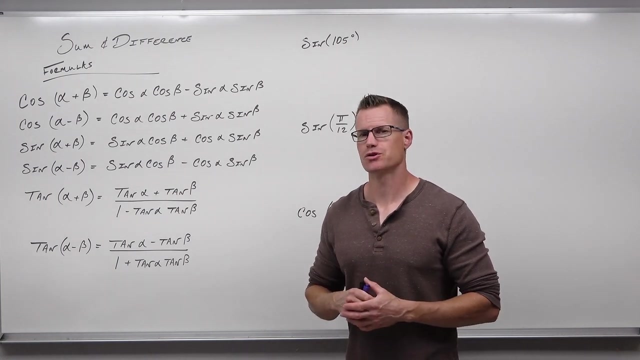 Hey there, welcome to another video. So in this video we're going to talk about some indifference formulas and, man, they look crazy but they're really useful. So a lot of times when we get angles that we want to find an exact solution for and it's not on a unit circle, this can help us.